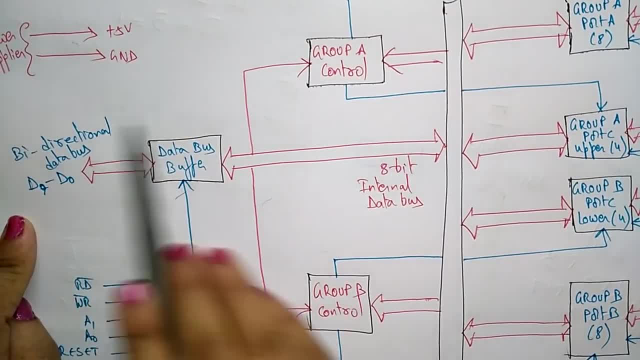 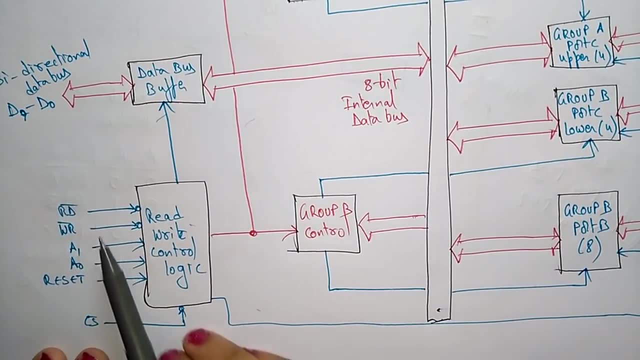 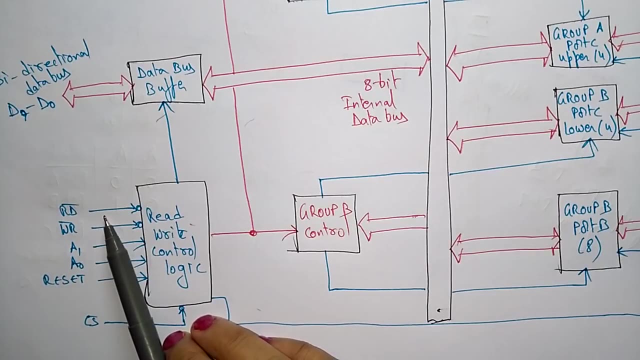 to 8255 and 8255 to CPU Only the data will be transferred here. And now, coming to the read or write control logic. This read- write control logic consisting of read signal, write signal A1, A0, reset and chip selection. So here the read. it reads the: 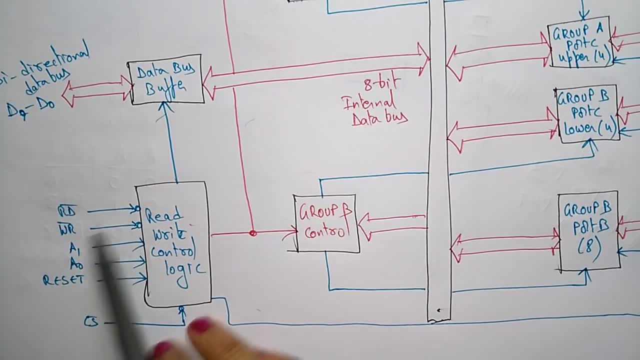 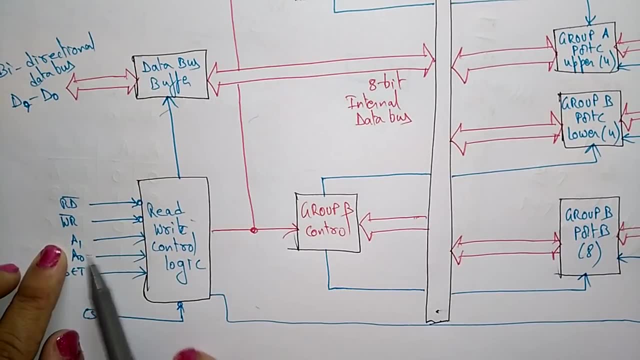 data from 8255 to the CPU and write the data from CPU to 8255, A0,, A1. So this indicates the port selection. So which port we have to be selected, either port A or port B or port C. So that will. 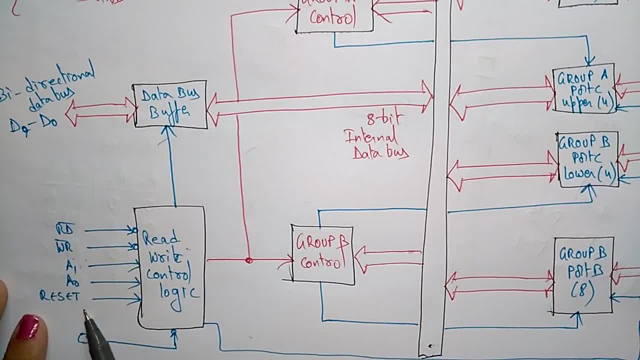 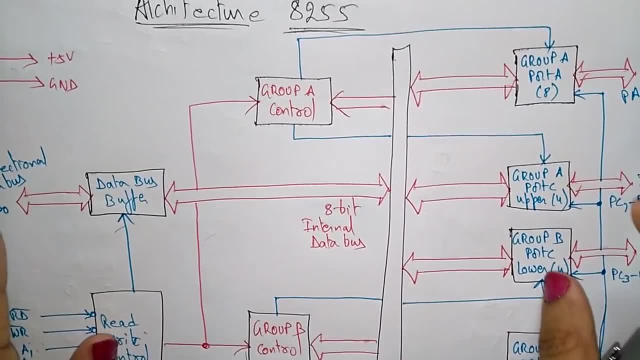 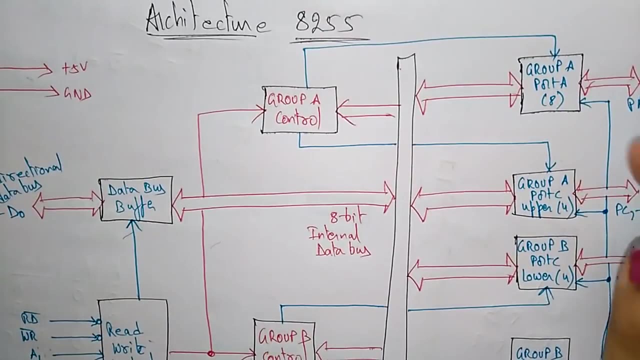 be two address bids, A0 and A1, and the reset. So these are all connected to read write control logic. Now coming to this, Actually this 8255 is divided into two groups, group A control and the group B control. So the group A control holds group A port A and group A port C upper. 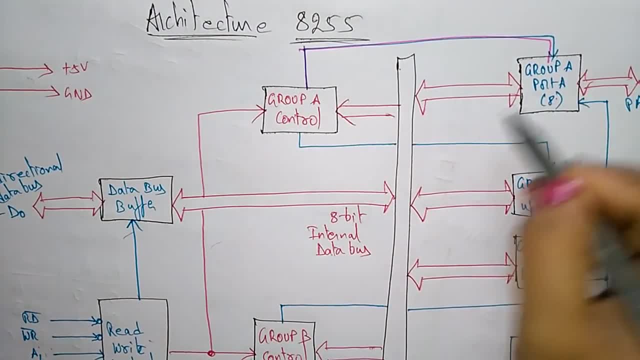 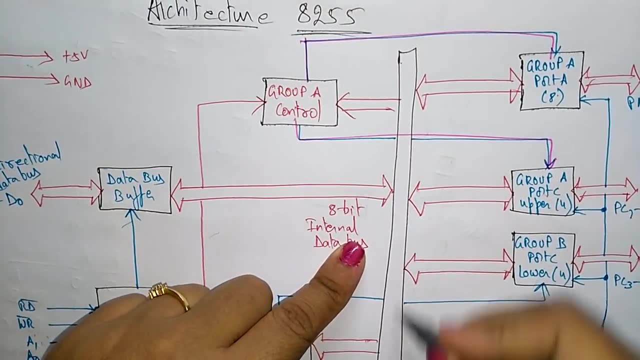 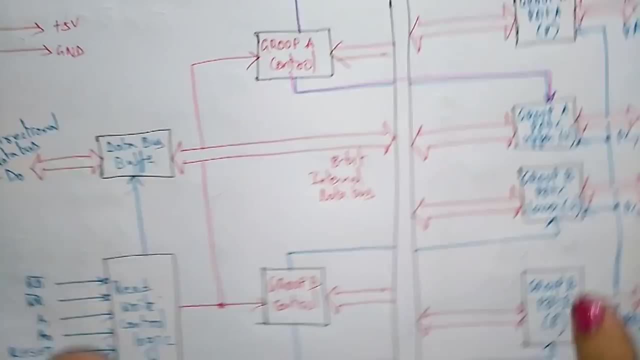 Okay, So this group A holds port A and port C upper. Okay, So this is an internal bus, So internal bus consisting of data bus, address bus and control bus. So this is the internal bus And here you have to be, remember that group. 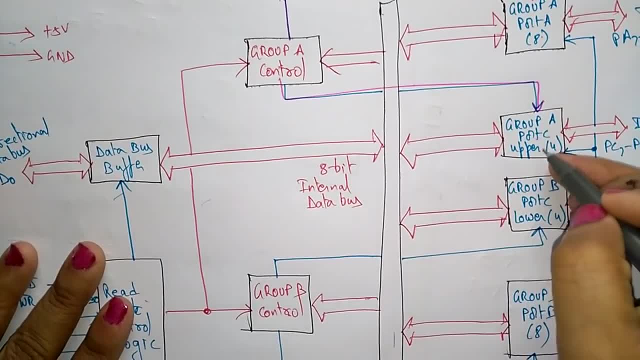 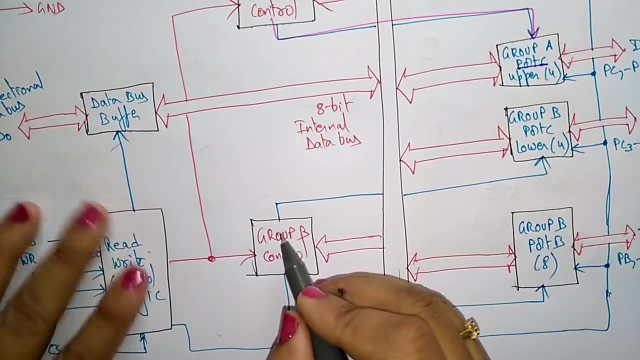 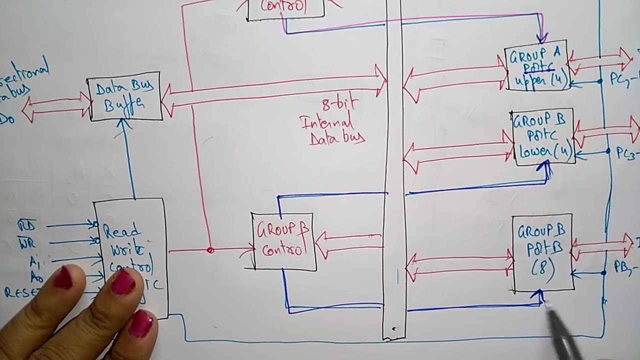 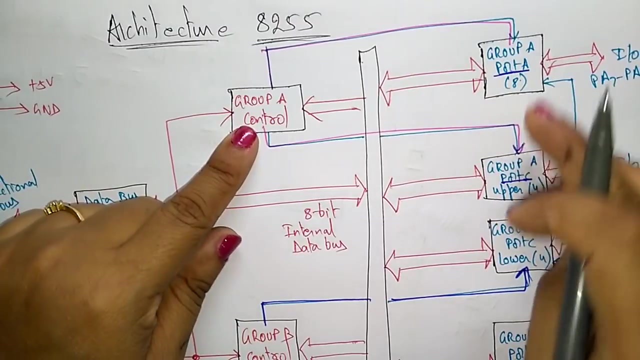 A control holds group A, port 8 bits and group A, port C, port A and port C upper, And whereas group B control holds port C lower and port B, Port B and port C lower, Group B- port C lower, port B, Group A- port A and group port C upper. 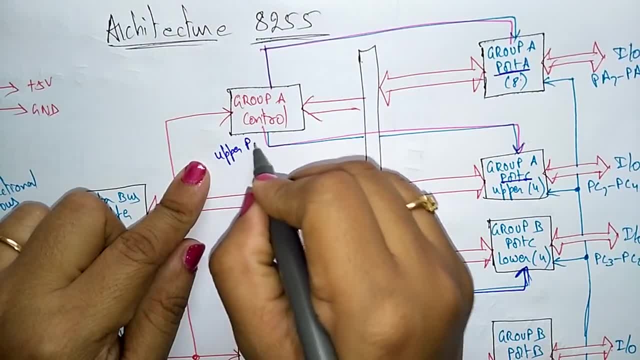 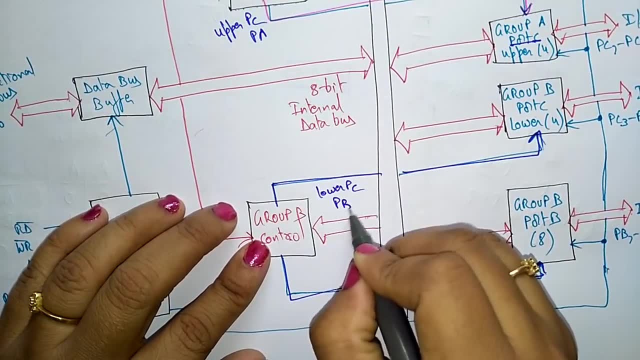 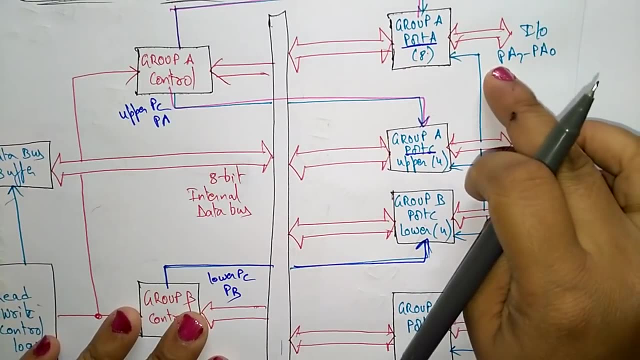 So you have to be remember that upper port C and port A, This group B consisting of lower port C and port B. Okay, And here you are. you are seeing that this is a input output pins, that is totally eight. eight pins are connected to the 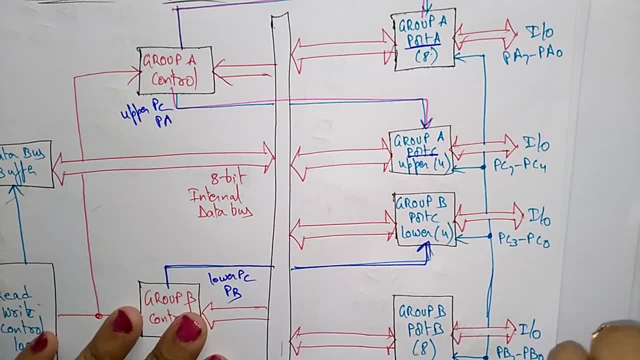 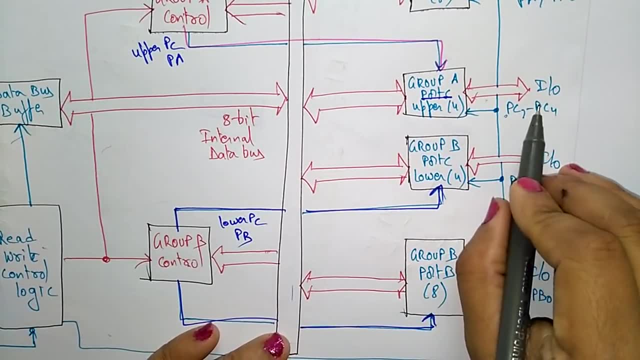 to the external devices. So you can take at a time you can take eight bits of information. Okay So, and here also this is the four bits are connected to input output devices And these are the four pins are connected to input output And this is a total eight bits, eight pins. 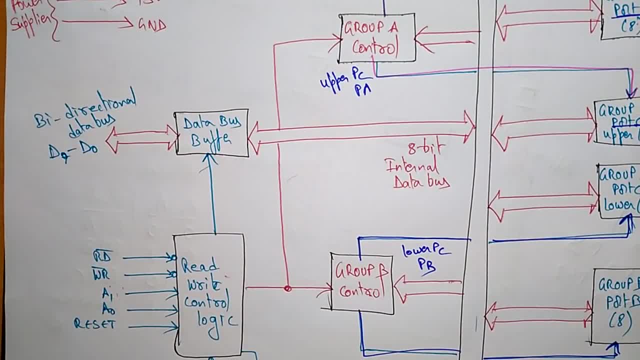 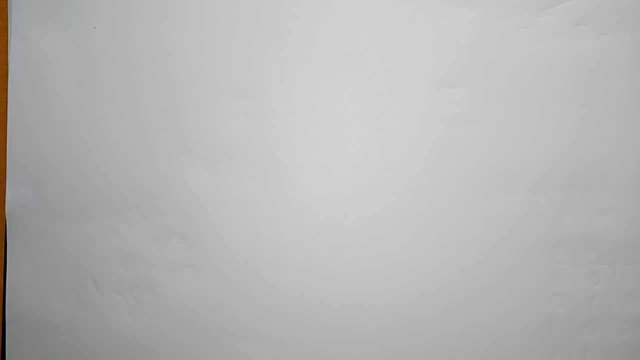 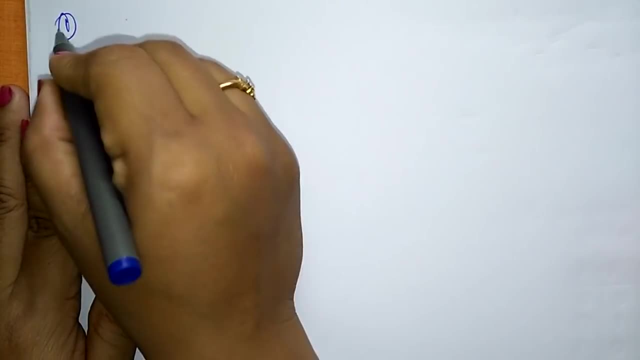 Now let us discuss each and every component clearly. The first we have to discuss about the data bus buffer. So what is this data bus buffer consisting of? Let me write that. So the this architecture, this complete eight, eight, two, double, five architecture, is divided. 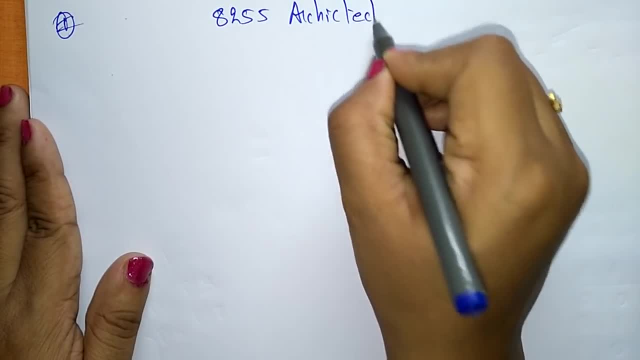 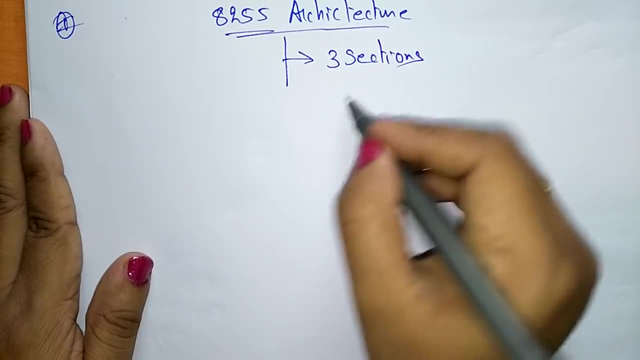 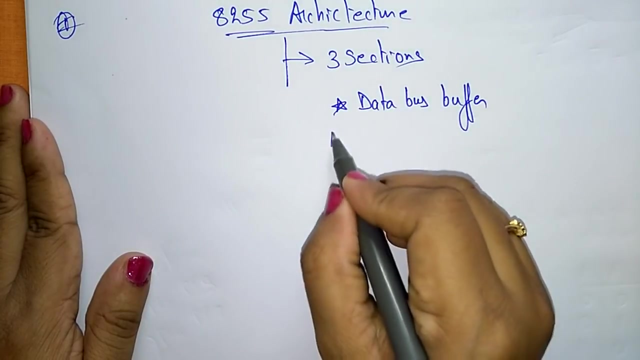 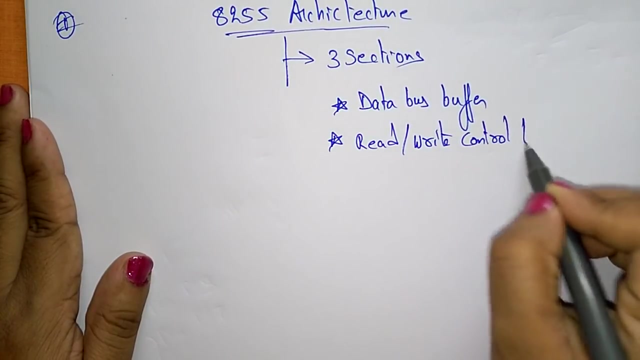 into three sections. Architecture is divided into three sections. So what are those? So first is data bus buffer. Next read write control logic, read write control logic. And the third one is group A and group B ports. Group A and 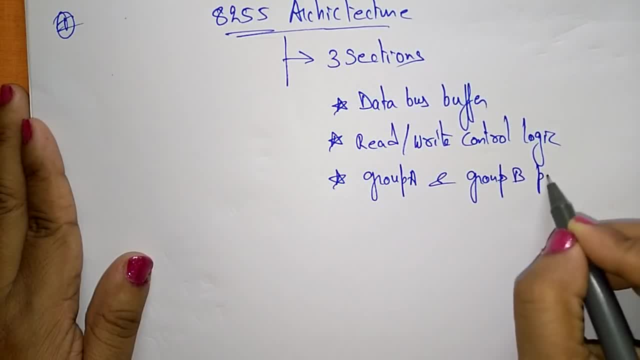 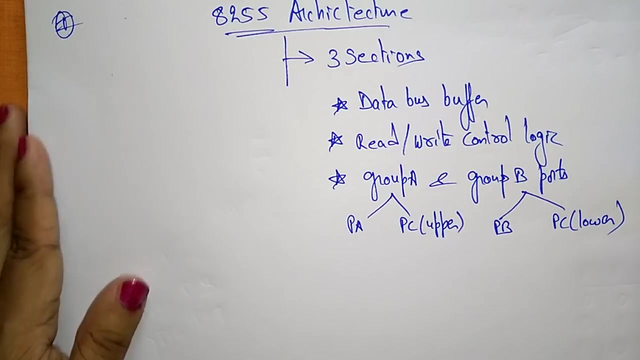 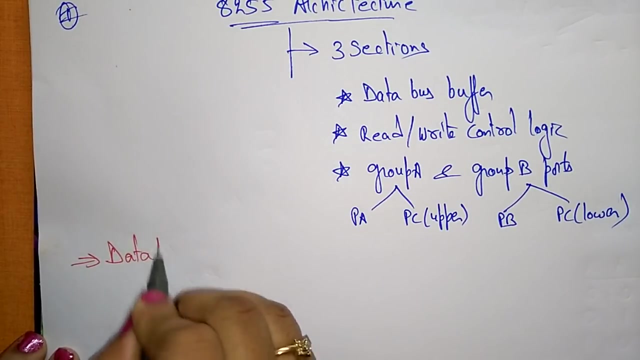 group B ports. So group A consisting of port A and port C upper, Group B consisting of port B and port C lower. Okay, So now this let us. what is this? port data bus buffer. Data bus buffer. 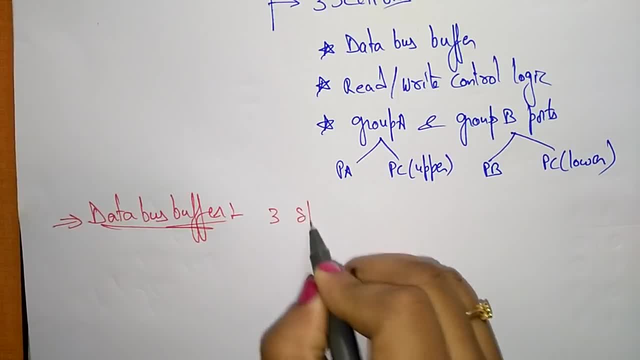 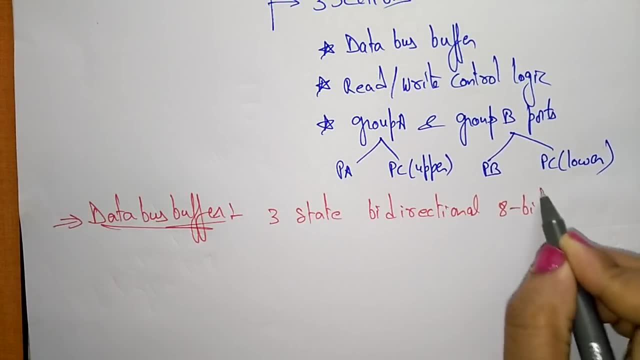 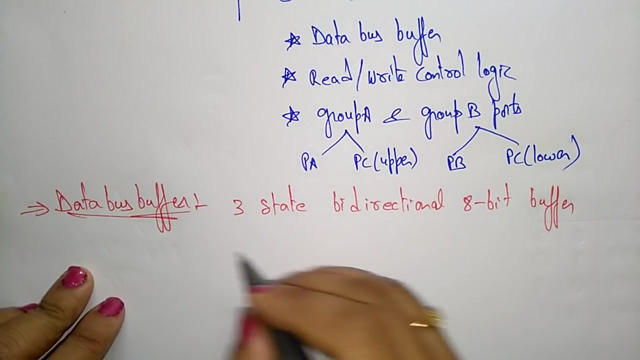 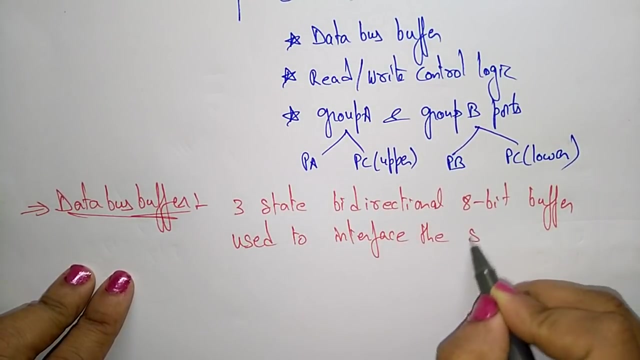 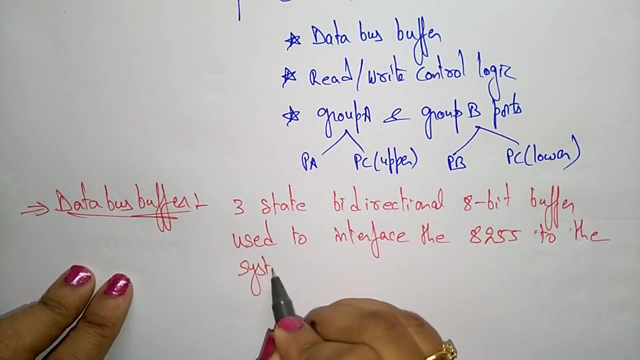 This data bus buffer is a first. it is a three-state, bi-directional, eight-bit eight-bit buffer. So data bus buffer is a three-state, bi-directional eight-bit buffer, user to interface, So users may connect this data to the system bus and update it. Knowledge. 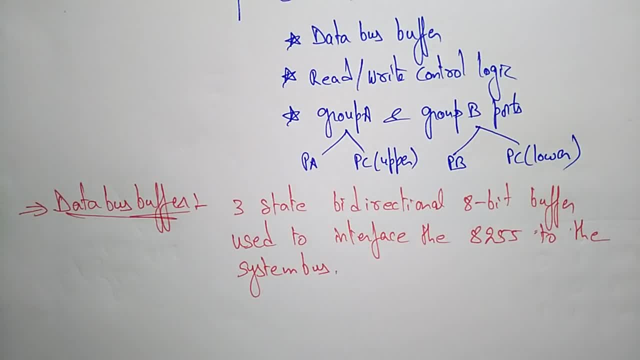 group users may always connect. So intelligence for some external resources, because cellular insider for any meaning is well subscribed to the data service, whether it is a dobroneg source, whether it is a server speech channel, PDD of some wireless, And that is item item, item item. 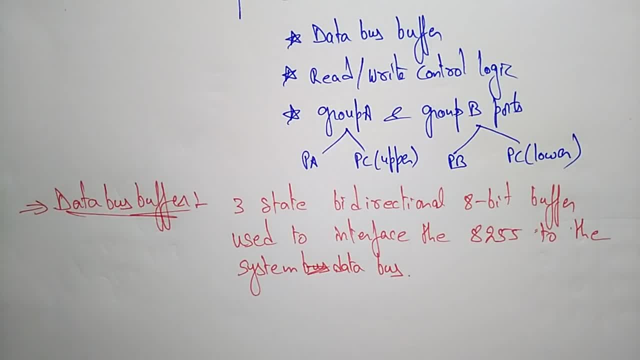 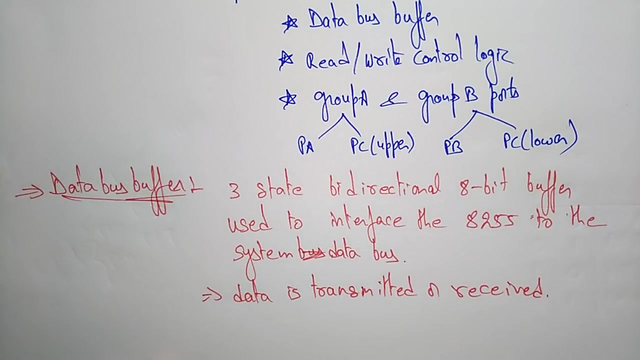 upon execution of input or the instruction by the CPU. so, whatever the instruction that the CPU is giving, based on that instruction the data is transmitted or received. the data is transmitted, transmitted or received based on the execution of the input, of input or instruction given by the CPU. 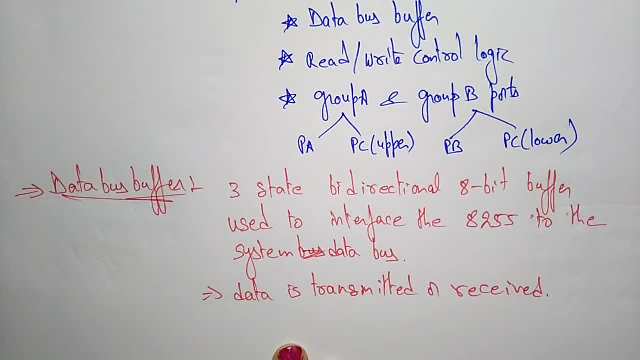 and here the control word or and status informations are also transferred through the data bus buffer. so here the control word or status information is also transferred, is transferred. so not only the data is transmitted or received, at the same time the control word or status information is also transferred. 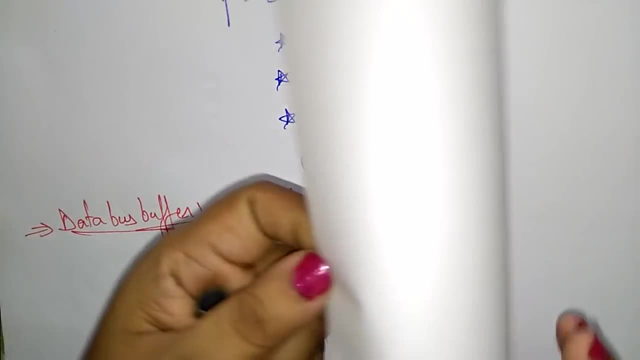 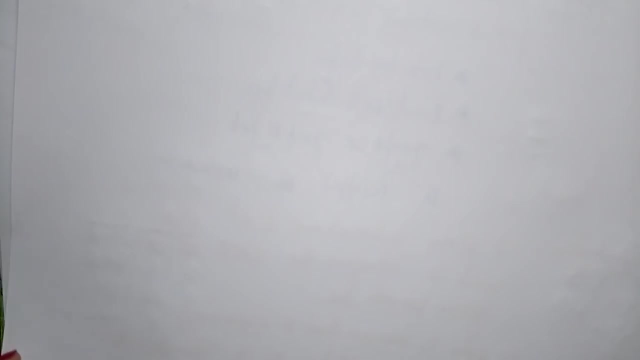 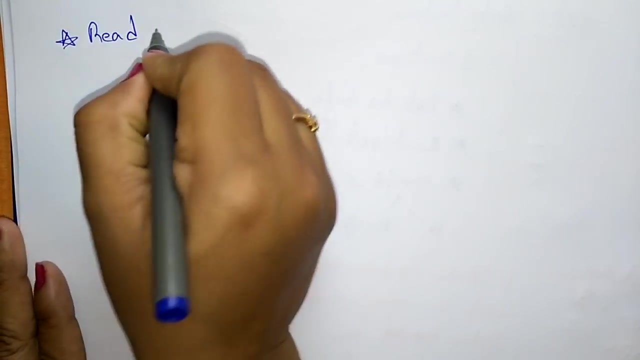 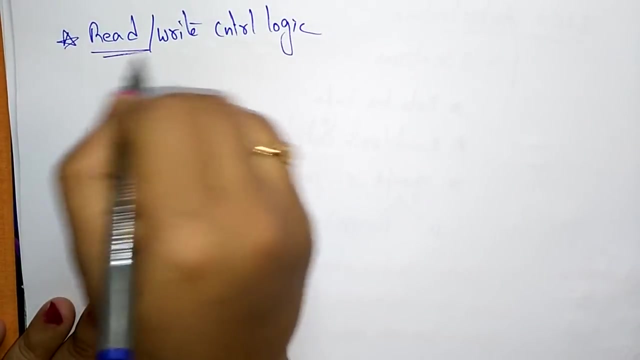 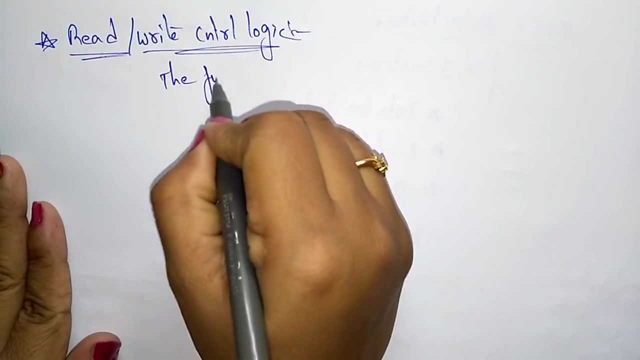 so this is about the data bus buffer. now let's go to the next slide. let us see what is this? read write logic. let me explain this: read write logic. read write, control logic. so what do we mean by this? read write. so the function, the function of this. 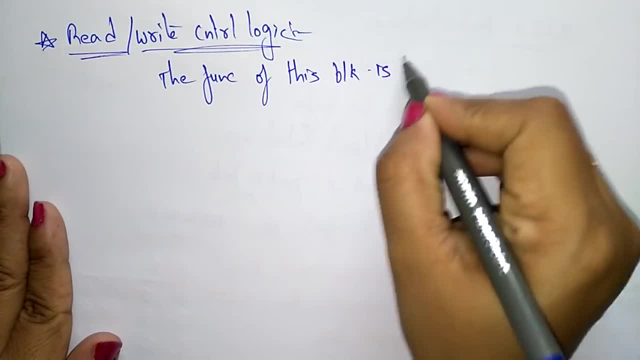 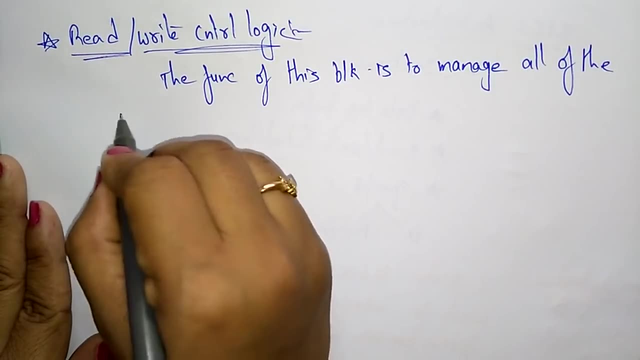 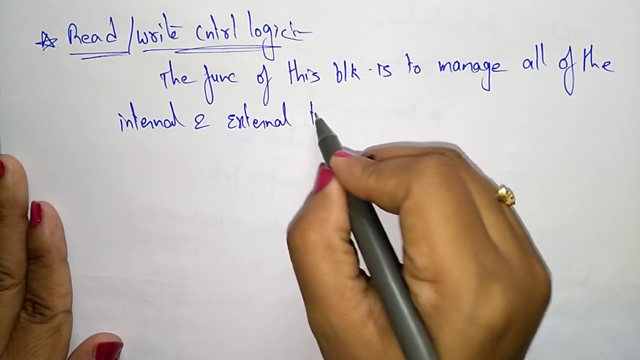 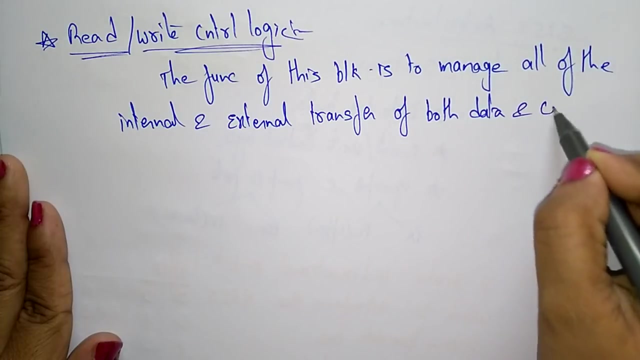 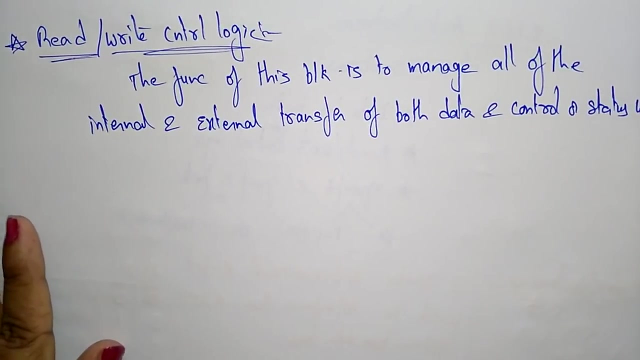 block is to manage. the main thing is is to manage all of the internal, internal and external transfer, transfer of both data and control or status words. so the main thing we have to do in this a25i to this CP and CP to 825 is we have 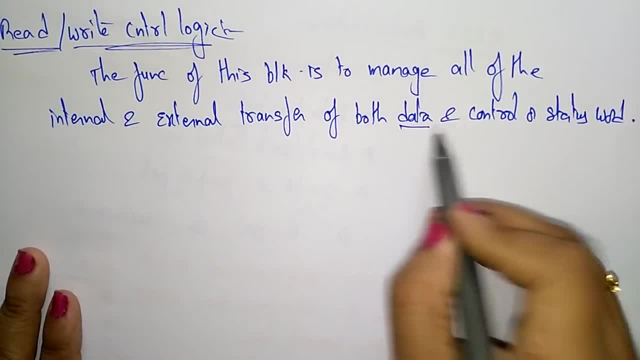 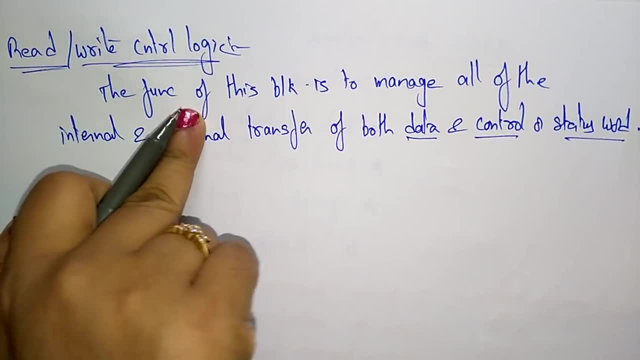 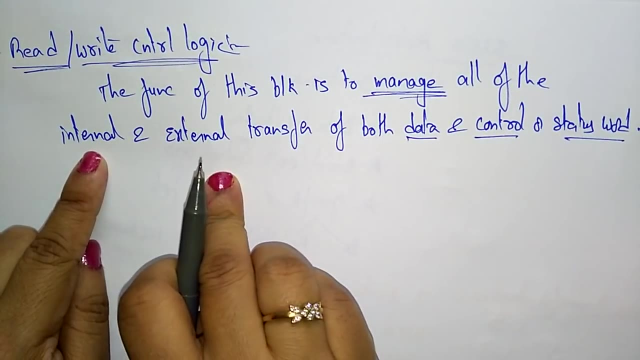 to transfer data, control or status point. so these 3 we have to be transferred. so this function of this block is to manage. it is going to be manage all of the internal and external transfers that are going from 8 to 5, 5 to 8, 08, 6 & 8, 0, 8, 6. 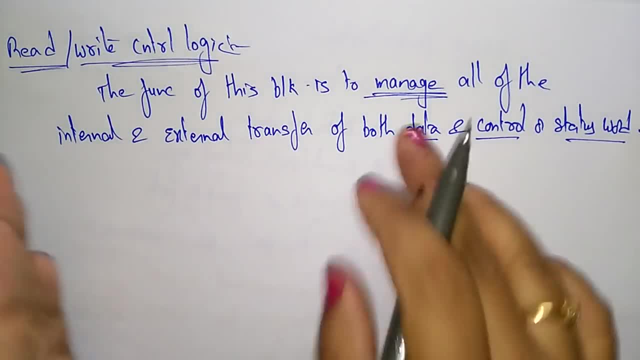 to 8255, so which are consisting ofzek where areатьwe have to be transferred these that are going from 8 to 5, 5 to 8086 and 8086- 28255, so which are consisting of data or control or status ports that will be managed by this. read write control logic. 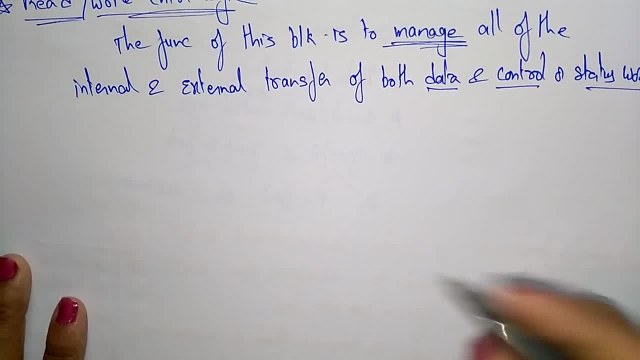 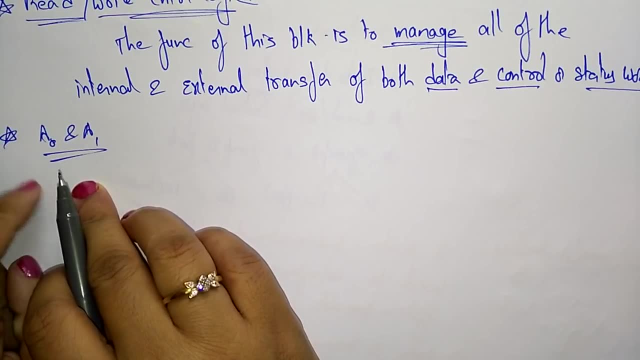 okay, so now let us see what is this: a0 and a1, a0 and a1 port. so i said this: a0 and a1. this is a port select 0 and a port select 1, so these input signals is conjunction with read and write chip. 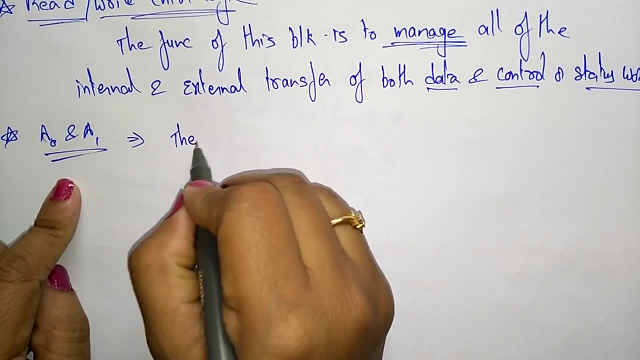 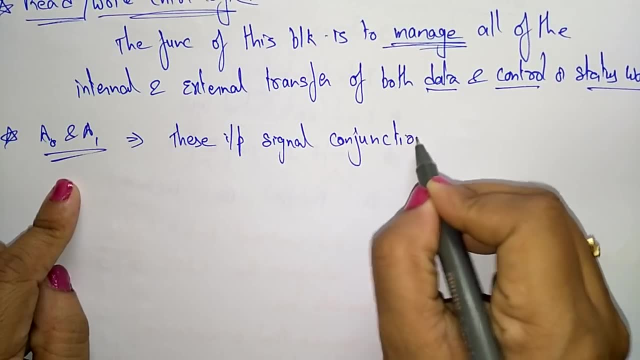 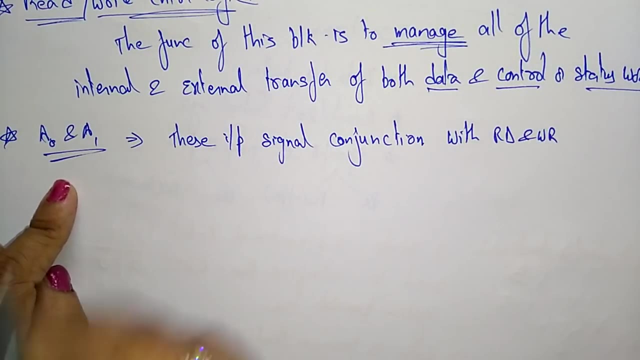 the first thing is the these input signal is always conjunction with conjunction with read, write. so when to read and when to write, and to which port we had to read and from which port we had to write, that will be decided by this a0 and a1 based on the chip selection. 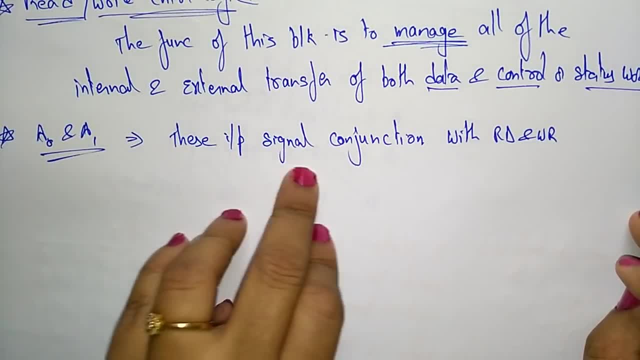 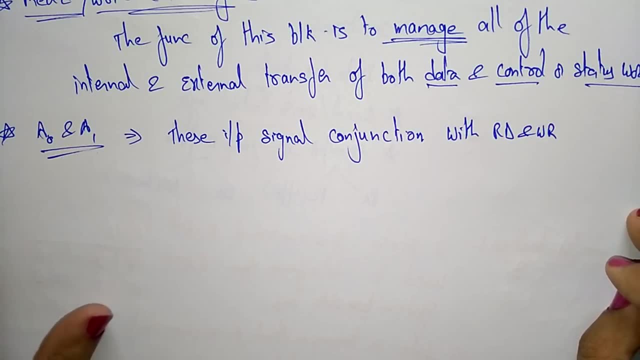 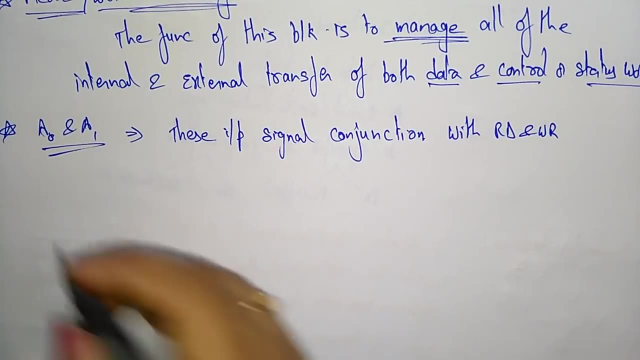 so this input signal, conjunction with read and write input, controls the selection of one of the three ports, ports uh, in this a255, and they are normally connected to the least significant bits of address, a0 and a1. so, and the next is a chip selection. so we know that the chip selection 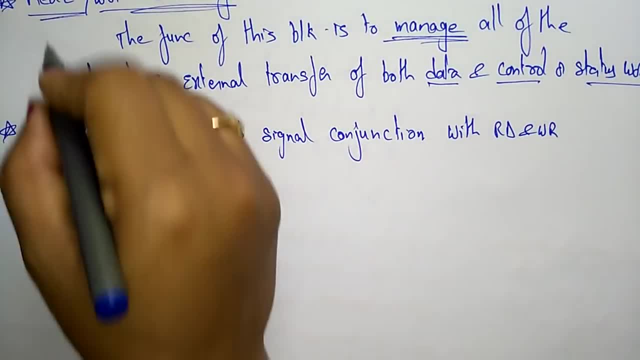 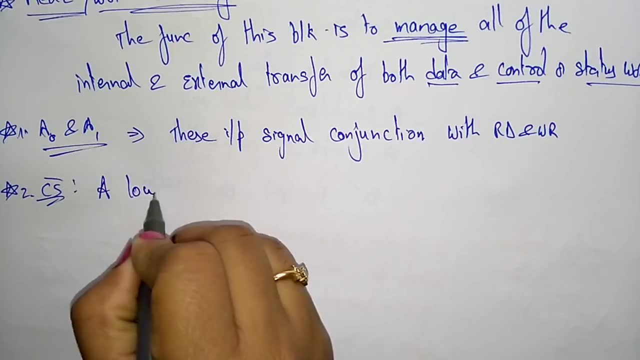 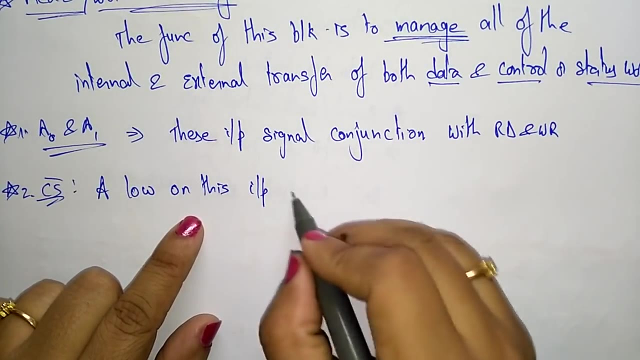 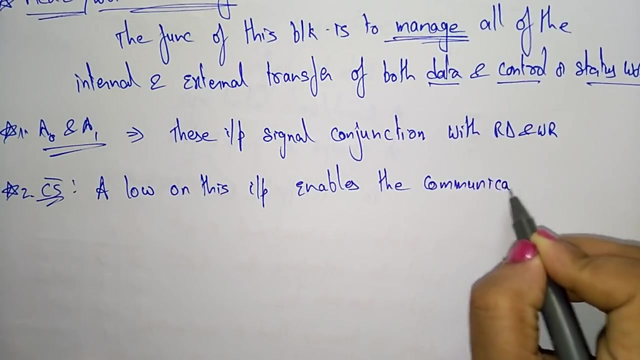 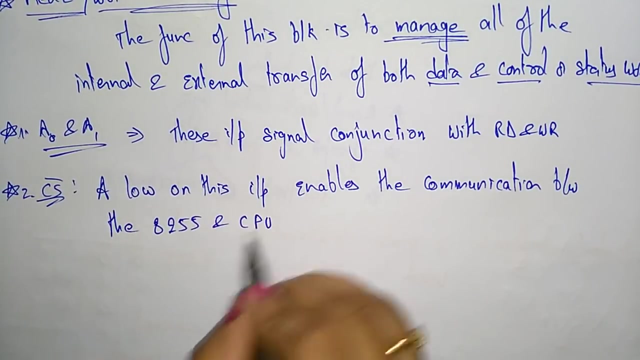 so these are all the pins connected that are present in the read write logic. okay, so these are present in read write logic. the chip selection: a low on this input. i already explained this about in pin diagram. a low on this input pin enables the communication between the a255 and cpu, so it is going to be enable the communication between a255. 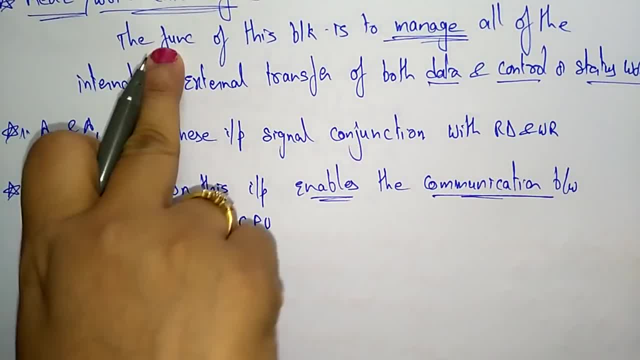 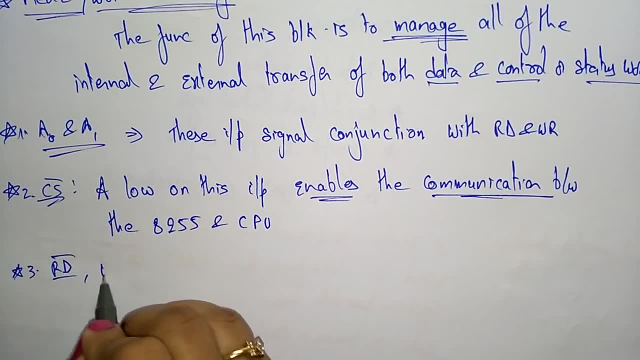 and the cpu. that will be done by the chip selection. so in read write control logic, you are having still uh rd bar. you are having still uh rd bar. you are having still uh rd bar and wr bar, so these are used for read, and and wr bar, so these are used for read and. 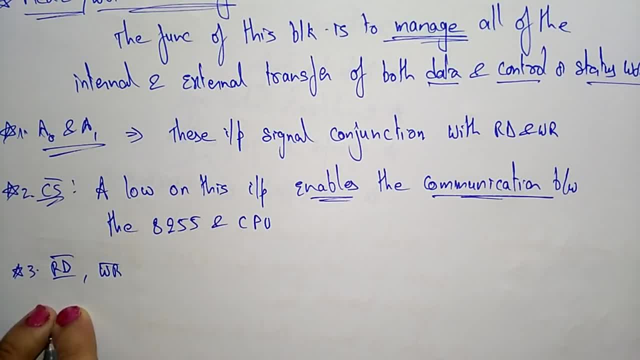 and wr bar. so these are used for read and write. so the read whenever a low on this. write. so the read whenever a low on this, write. so the read whenever a low on this. pin enables 8258255 to send the data or. pin enables 8258255 to send the data or. 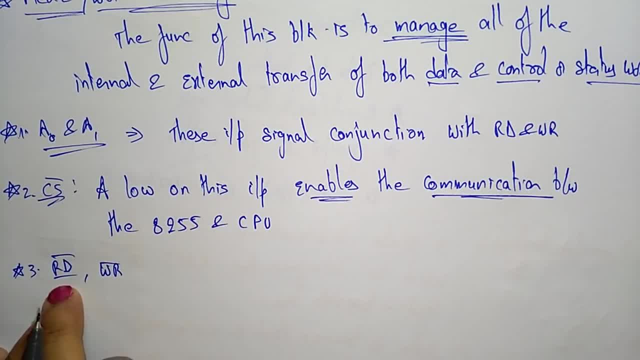 pin enables 8258255 to send the data or status information to the cpu. status information to the cpu. status information to the cpu. okay, it is going to be send the data. or okay, it is going to be send the data. or okay, it is going to be send the data or status information to cpu. 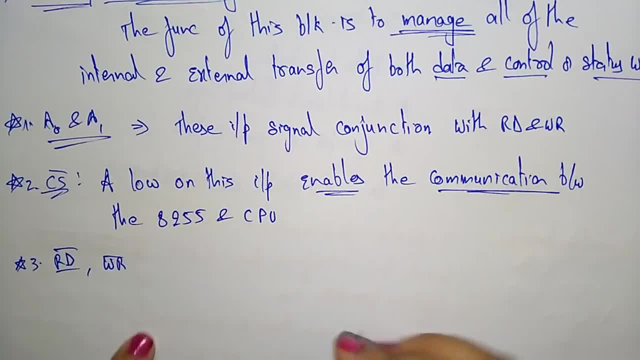 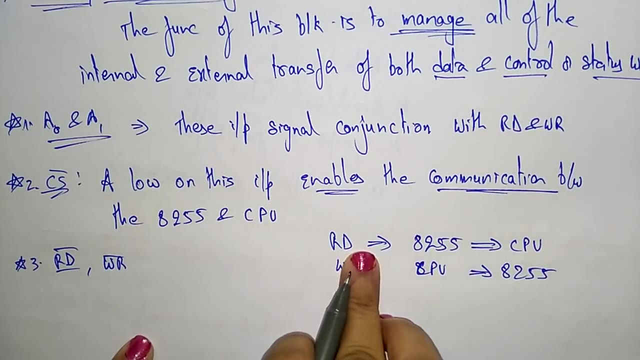 status information to cpu. status information to cpu. where as write signal from cpu to 8255, where as write signal from cpu to 8255, So read is 8255 to CPU and whereas write is CPU to 8255.. We are reading the data from 8255 to CPU and write is performing the data is returning to the 8255. 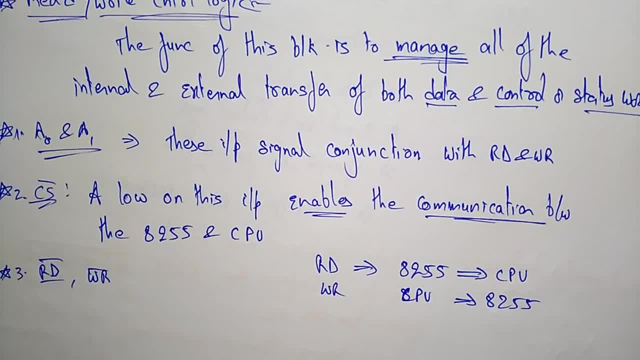 Okay, and the next component, next section, is the group A and group B controllers, So that we will discuss in the next video. Thank you, Thank you.